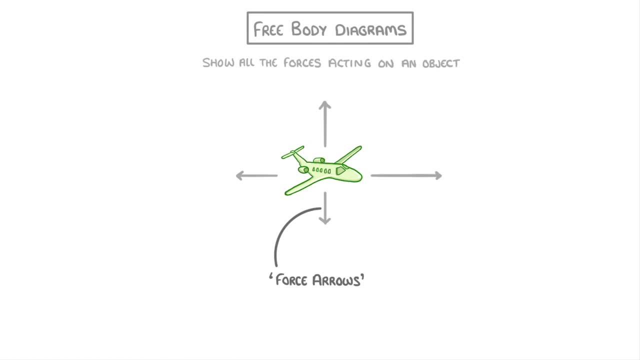 do this using force arrows. So if we took the example of a plane flying through the sky, we would draw its free body diagram by adding a bunch of different arrows that represent all the forces acting on the plane, So we'd have one going forwards, which would be its. 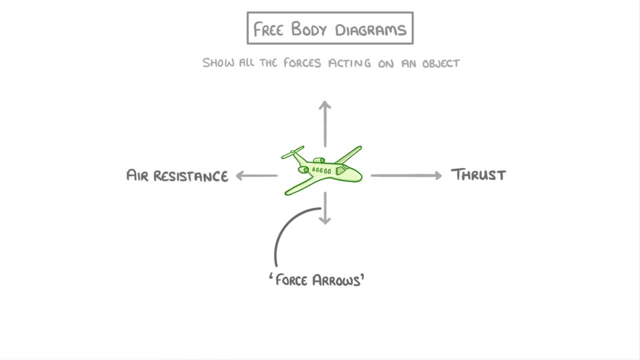 thrust one backwards for air resistance, or drag one downwards for its weight and one upwards for its lift. Because all forces are vectors, each of these has to have both a magnitude and a direction. We can see the direction from which way the arrows are pointing, but the magnitude of 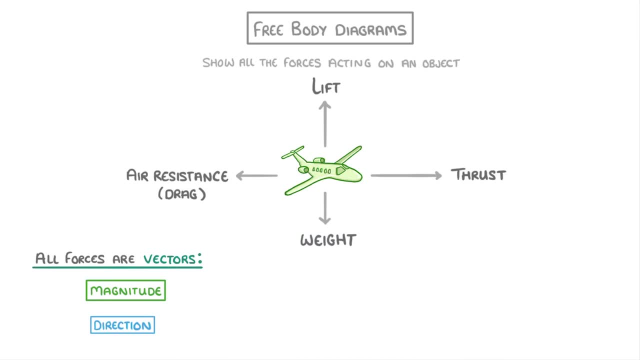 the force comes from, how long each of the arrows are And, to be more precise, we can label each of them in newtons. Now, because all these forces are acting in different directions, some of them are going to cancel each other out, And once we've taken that into account, what we'd have left? 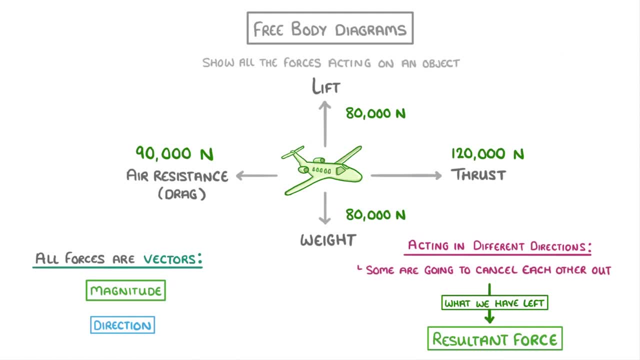 is the resultant force, which we can describe as the overall force on an object. It's normally easiest to do this by looking at the horizontal and vertical directions separately and calculating the overall size and direction of the resultant force in each case. For example, the vertical component is the resultant force on an object and the horizontal 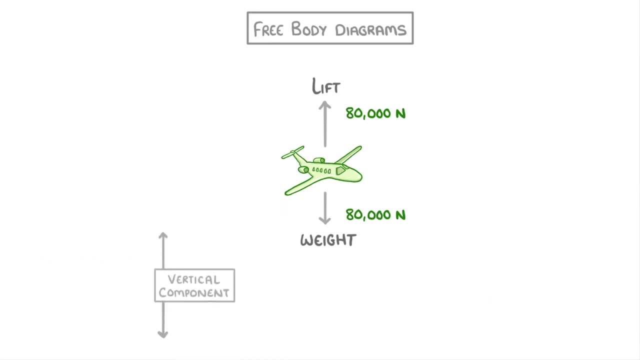 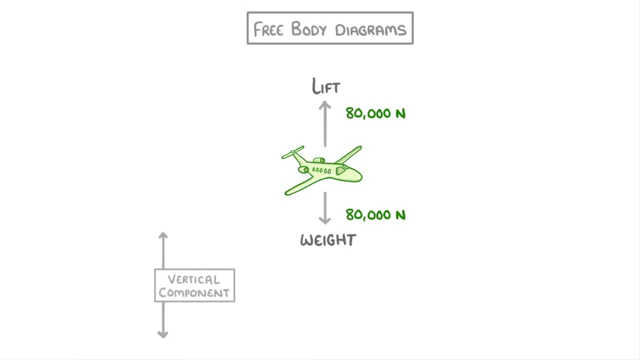 The vertical component of this free body diagram involves a force of 80,000 Newtons up and 80,000 Newtons down, So when we subtract one from the other, we're left with zero Newtons overall for the vertical component. For the horizontal component, though, we have 120,000 Newtons to the right and only 90,000. 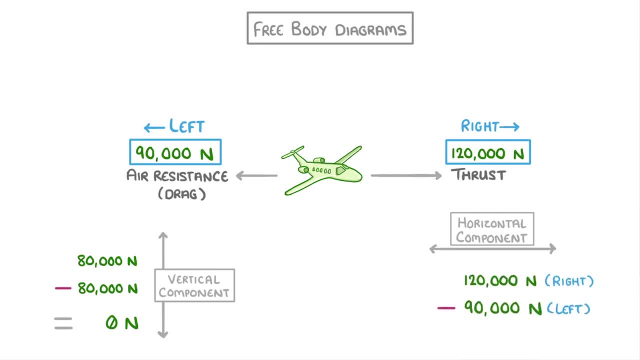 Newtons to the left. So by doing right minus left, we get the resultant force on the vertical, we get a resultant force of 30,000 newtons in the right direction. So overall, taking into account the vertical and horizontal components, we'd still have an overall resultant force of 30,000 newtons to the right.